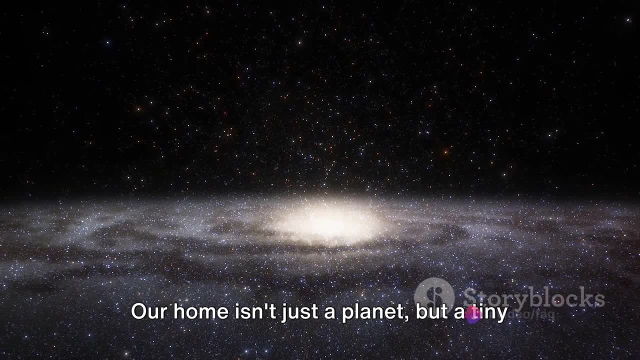 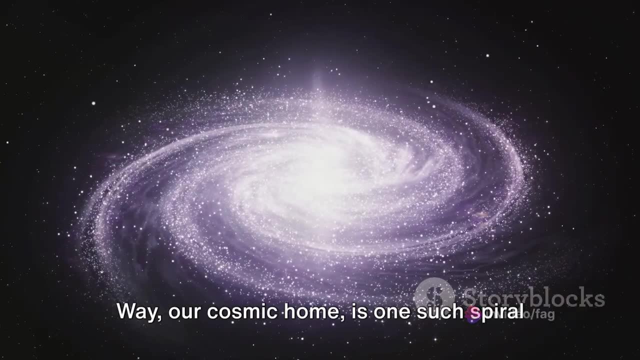 It's an awe-inspiring thought, isn't it? Our home isn't just a planet, but a tiny part of a grand cosmic dance that's been going on for billions of years. The Milky Way, our cosmic home, is one such spiral galaxy, a celestial wonder that we're 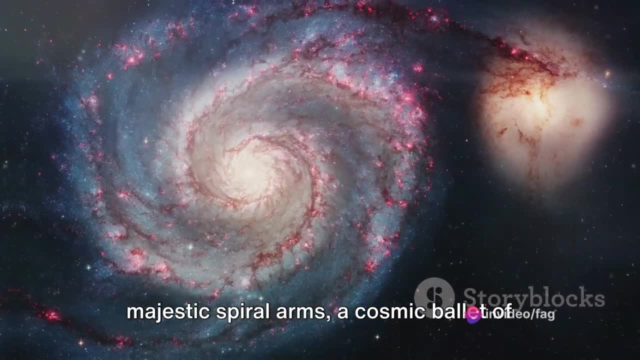 about to explore. At the heart of our galaxy lie the majestic spiral arms, a cosmic ballet of stars and galaxies. The Milky Way, our cosmic home, is one such spiral galaxy, a celestial wonder that we're about to explore. At the heart of our galaxy lie the majestic spiral arms, a cosmic ballet of stars and galaxies. 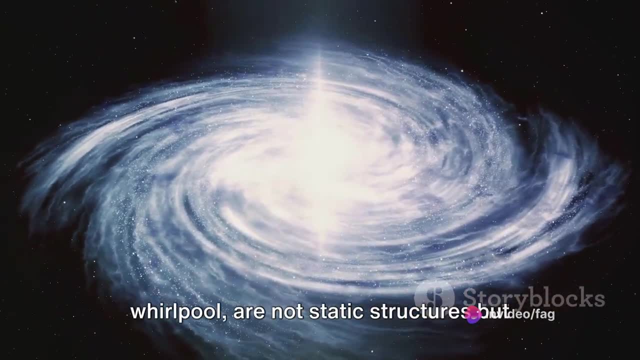 The Milky Way, our cosmic home, is one such spiral galaxy, a celestial wonder that we're about to explore. At the heart of our galaxy lie the majestic spiral arms, a cosmic ballet of stars and galaxies. These arms, like a grand cosmic whirlpool, are not static structures but dynamic. 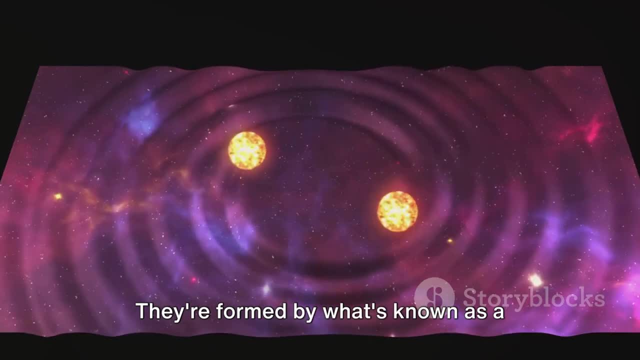 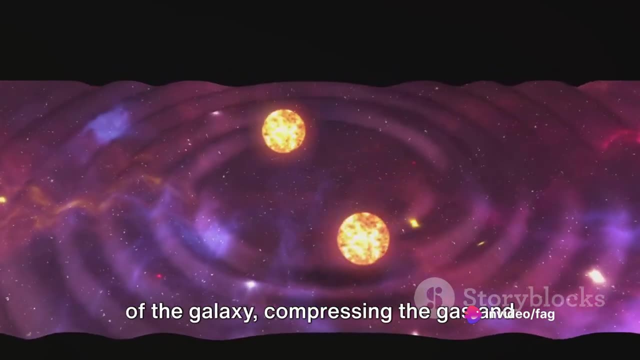 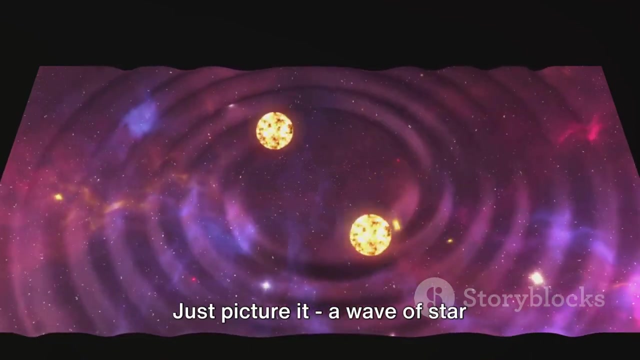 constantly shifting and evolving entities. They're formed by what's known as a density wave, a gravitational perturbation that travels through the disc of the galaxy, compressing the gas and dust in its path and triggering the birth of new stars. Just picture it: a wave of star formation rippling out across the galaxy. 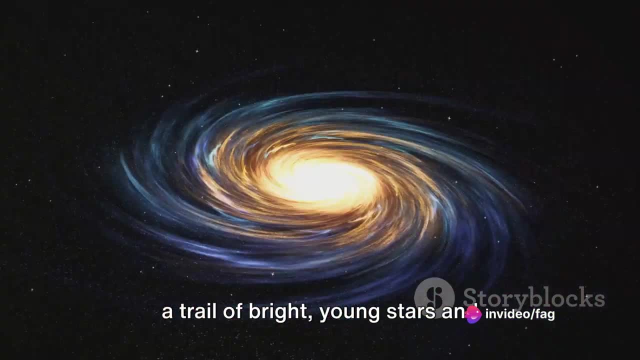 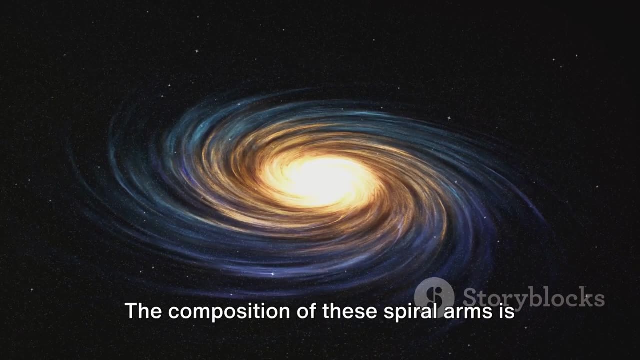 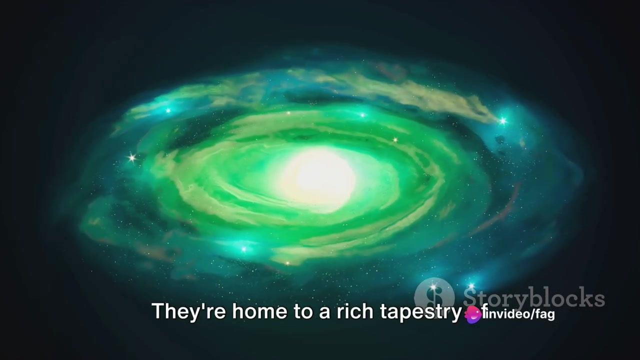 And as this wave passes, it leaves behind a trail of bright young stars and nebulous gas clouds, creating the intricate spiral pattern we associate with galaxies like our own. The composition of these spiral arms is as fascinating as their formation. They're home to a rich tapestry of 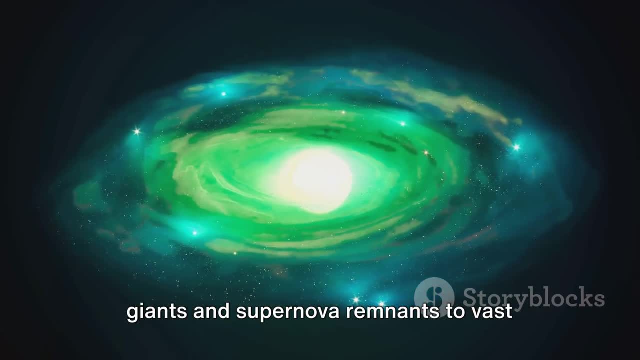 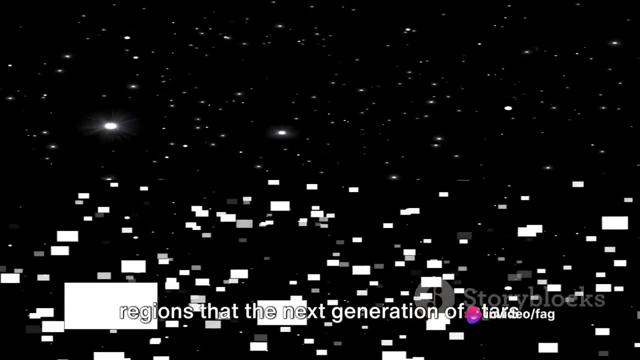 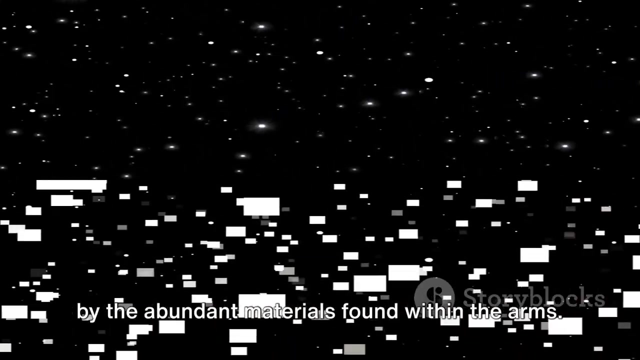 celestial objects, from luminous blue giants and supernova remnants to vast nebulae and clusters of young stars, And it's within these dense, gaseous regions that the next generation of stars and planetary systems are born, nurtured by the abundant materials found within the arms. 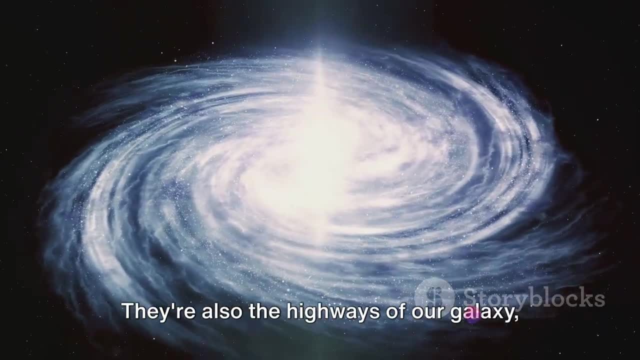 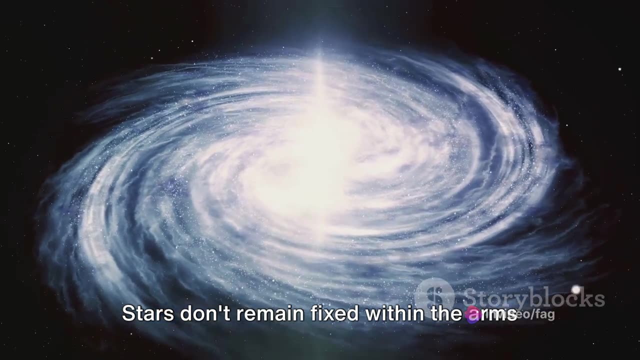 Yet the spiral arms are more than just stellar nurseries. They're also the highways of our galaxy, guiding the motion of stars and gas as they orbit the galactic center. Stars don't remain fixed within the arms, but move in and out of them as they travel along their paths. 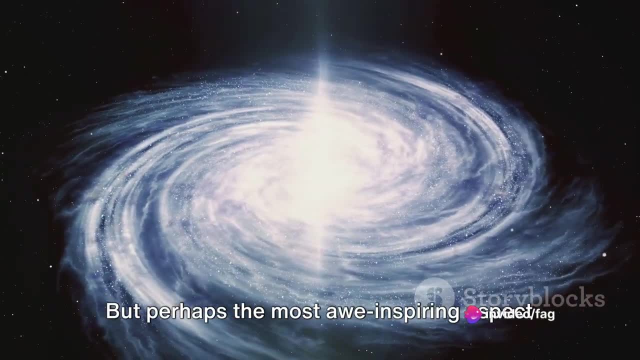 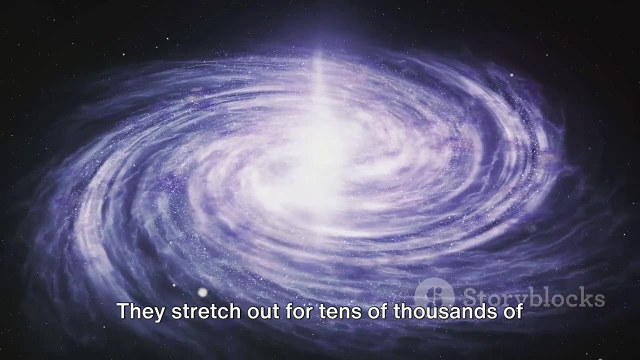 resulting in the beautiful and intricate patterns we observe. But perhaps the most awe-inspiring aspect of the Milky Way's spiral arms is their scale. They stretch out for tens of thousands of light years, weaving their way through the galactic disk in a grand dance that has been 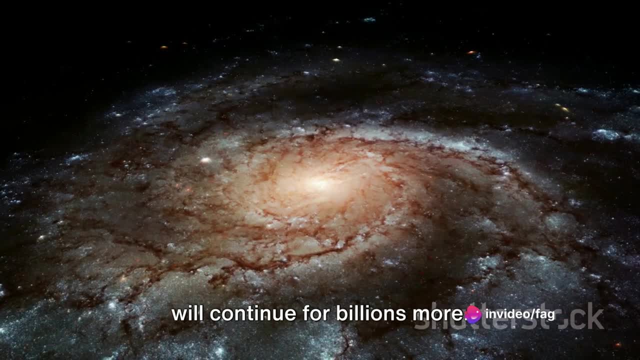 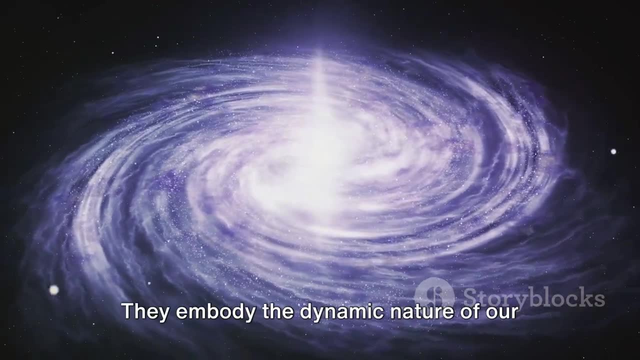 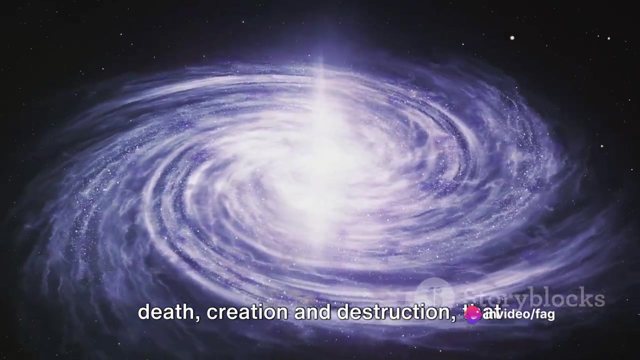 ongoing for billions of years and will continue for billions more. These arms, with their swirling patterns, are more than just beautiful. They are the cradle of new stars. They embody the dynamic nature of our galaxy, the constant cycle of birth and death, creation and destruction. 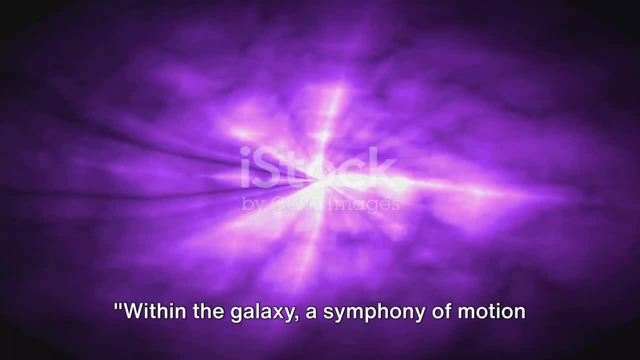 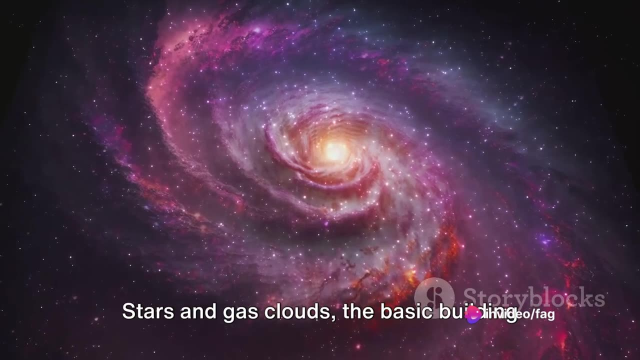 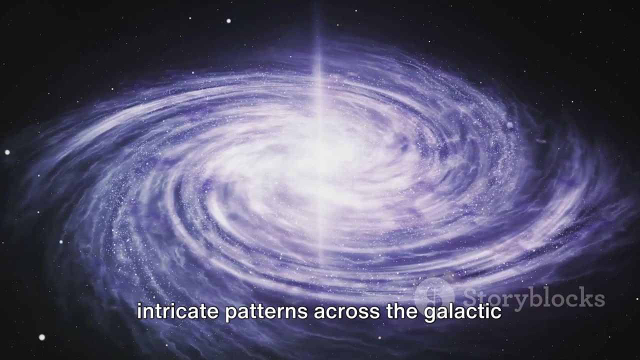 that shapes the universe we inhabit. Within the galaxy, there is an endless cycle of motion that plays out, orchestrated by the unseen hand of gravity. Stars and gas clouds, the basic building blocks of the Milky Way, are constantly on the move. Their paths, known as orbits, trace out intricate patterns across the galactic disk. 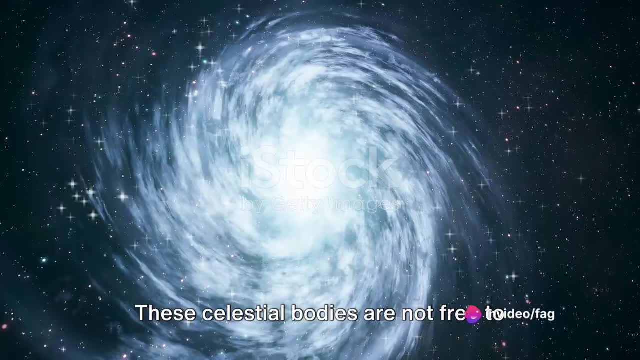 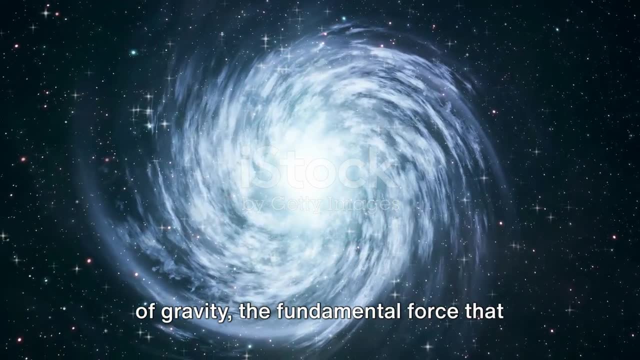 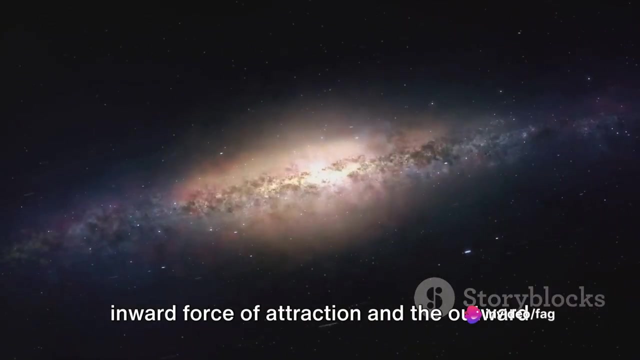 creating a dynamic tapestry of motion that changes over millions of years. These celestial bodies are not free to wander at will. Instead, they are bound by the iron grip of gravity, the fundamental force that shapes the structure of the galaxy. Gravity pulls everything together, creating a delicate balance between the inward force of 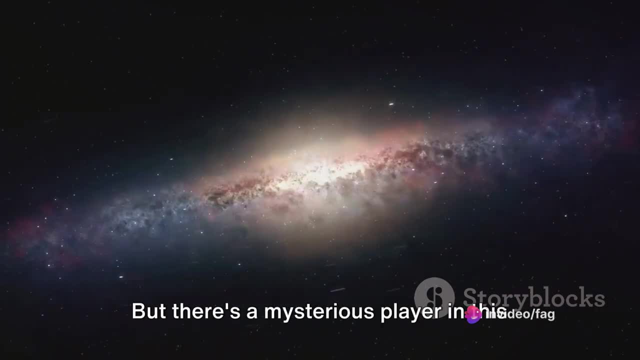 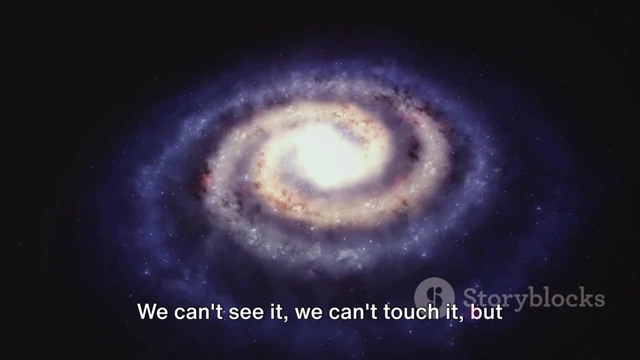 attraction and the outward motion of the stars and gas. But there's a mysterious player in this cosmic ballet: dark matter. We can't see it, we can't touch it, but we know it's there because of the way it influences the motion of stars and gas. 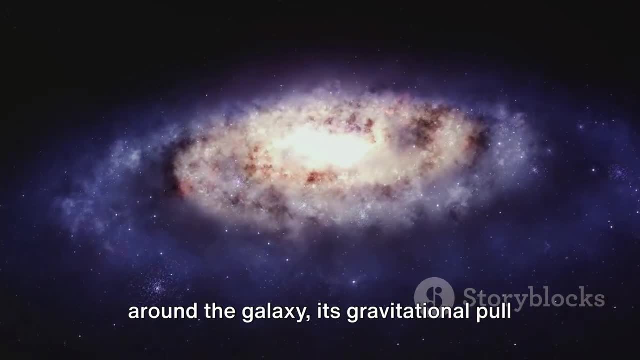 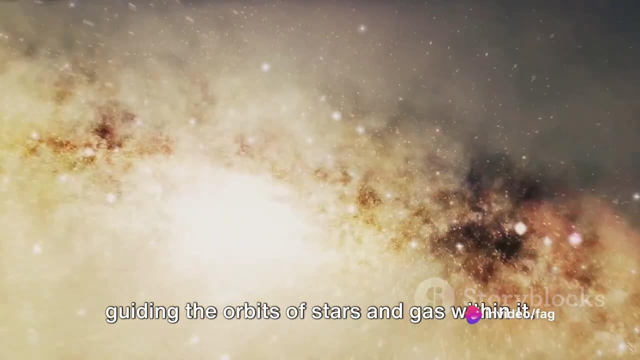 Dark matter forms a vast invisible halo around the galaxy, its gravitational pull helping to hold the Milky Way together and guiding the orbit of the galaxy. It's a complex dance, but one that's essential for the structure and evolution of the galaxy. 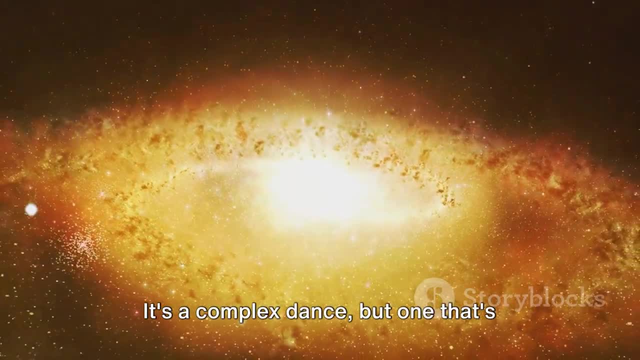 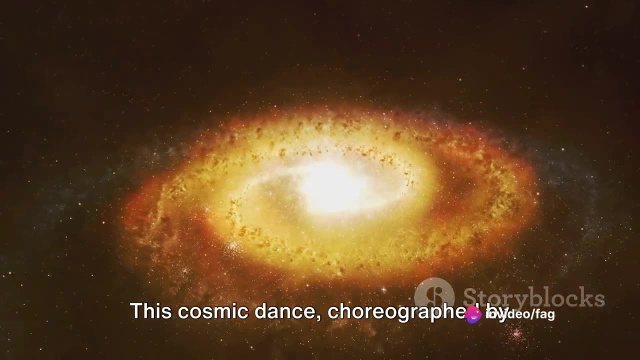 This cosmic dance, choreographed by gravity, shapes the galaxy as we know it. The Milky Way is a diverse neighborhood home to stars of all ages and sizes. In this celestial city, the bustling spiral arms are the cradles of youth where hearts 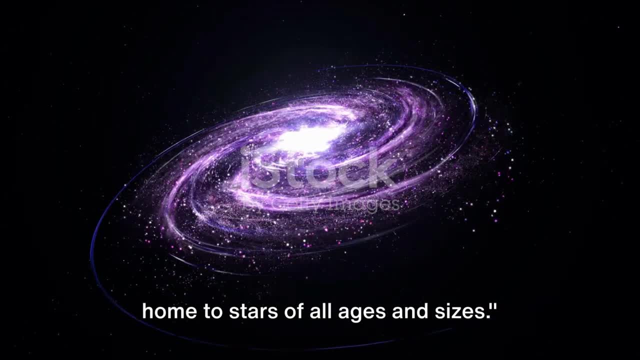 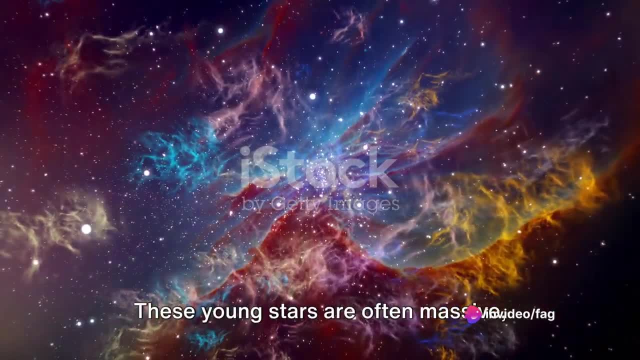 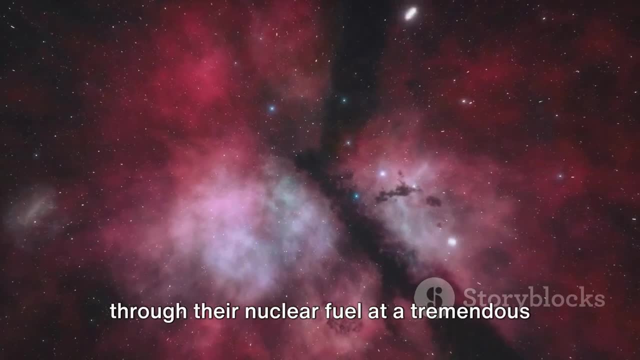 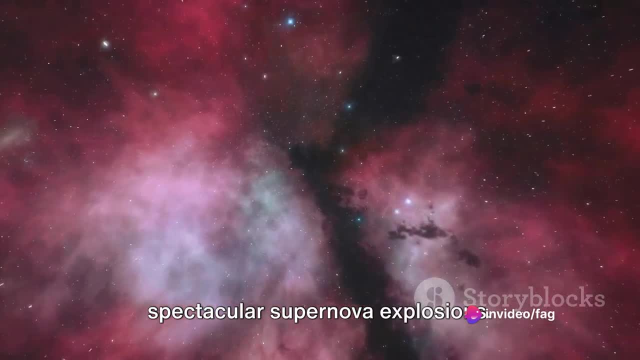 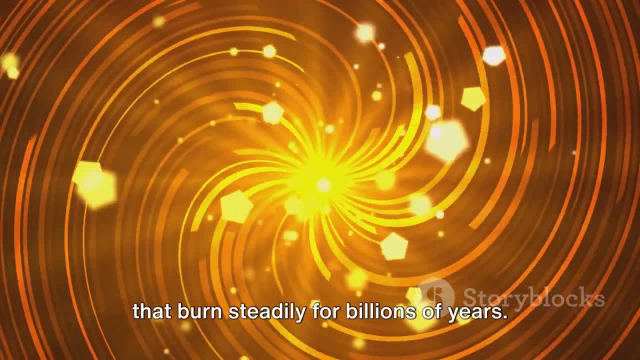 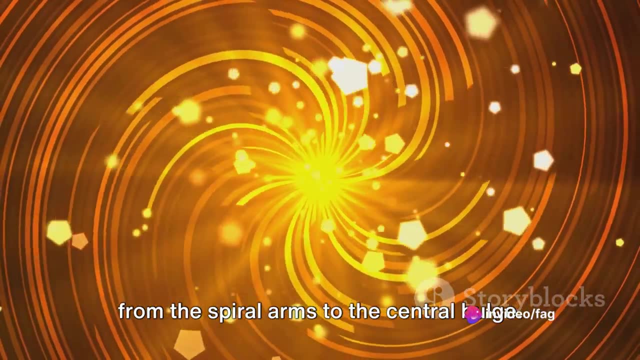 Love is the ground we set about. Vłaščarė New yıl phones, Star Mirror, Planeta, Moon, ��자 KK Universe. Very Glorious Ji-Go dialogu ион. Then there are the seniors of our galactic neighborhood, the ancient dim stars. 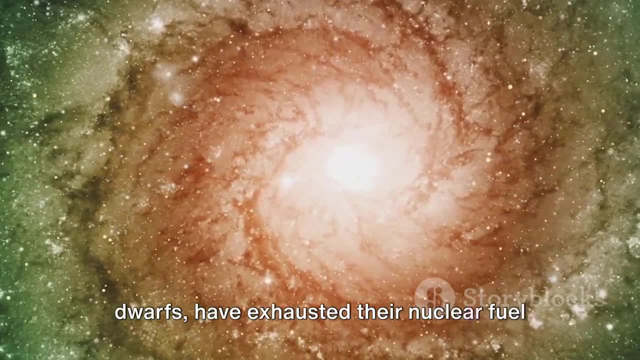 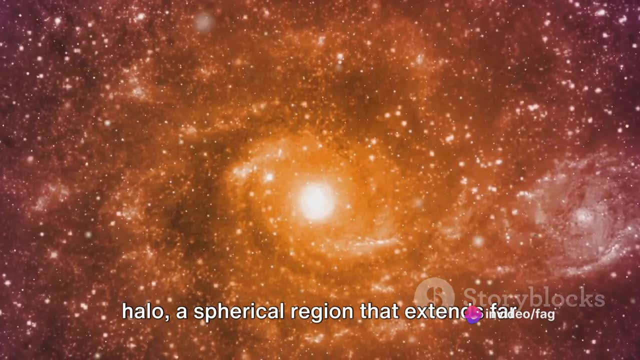 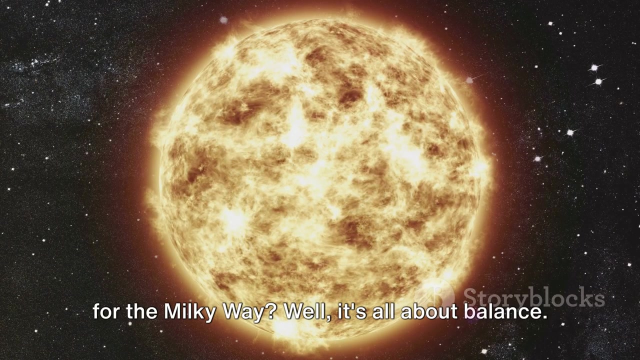 These stars, often red giants or white dwarfs, have exhausted their nuclear fuel and are in the last stages of their lives. They are typically found in the galactic halo, a spherical region that extends far beyond the galaxy's visible disc. But what does this stellar diversity mean for the Milky Way? 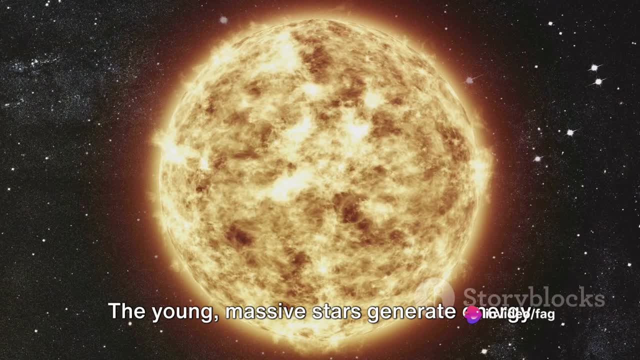 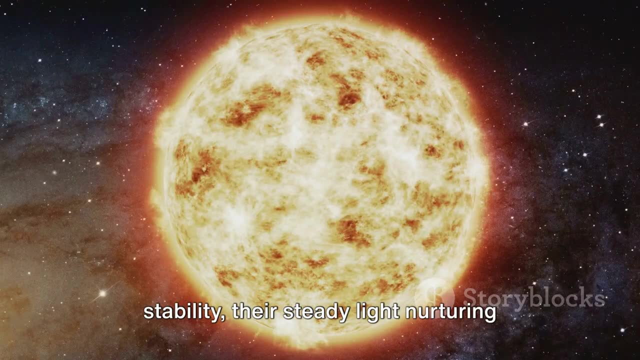 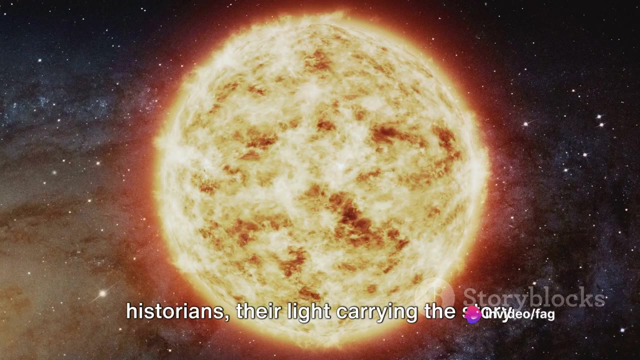 Well, it's all about balance. The young massive stars generate energy and elements essential for life. The mature stars, like our sun, provide stability, their steady light nurturing life on planets that orbit them. And the ancient stars? they are the historians, their light carrying the story of our galaxy's. 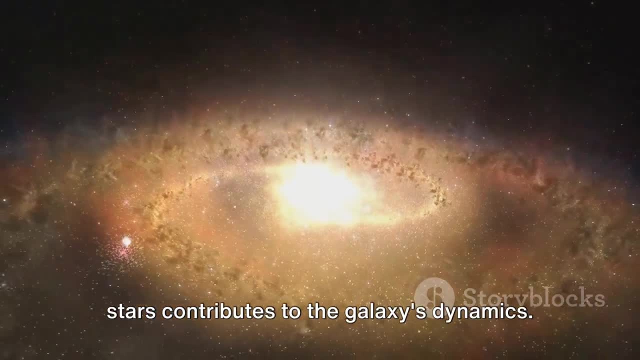 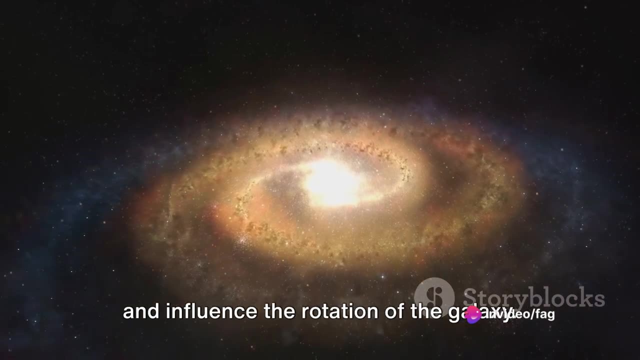 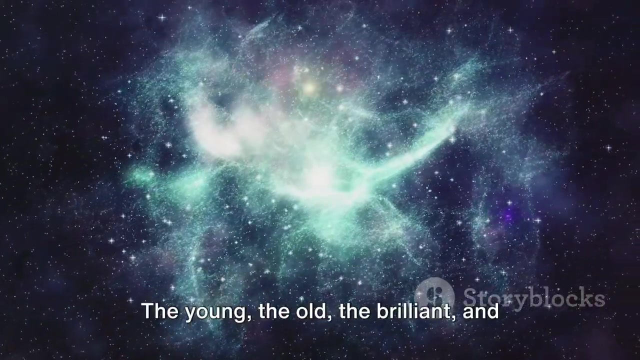 past. Furthermore, the distribution of these stars contributes to the galaxy's dynamics. The mass of the stars and their motion, governed by gravity, shape the spiral arms and influence the rotation of the galaxy. So, in the grand scheme of our Milky Way, every star matters. 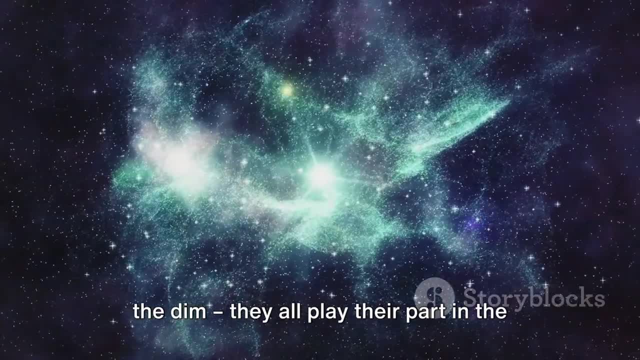 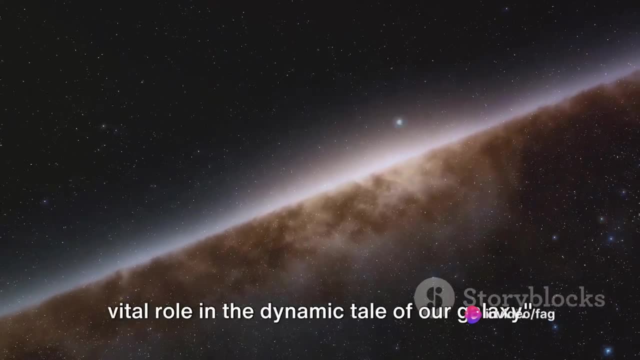 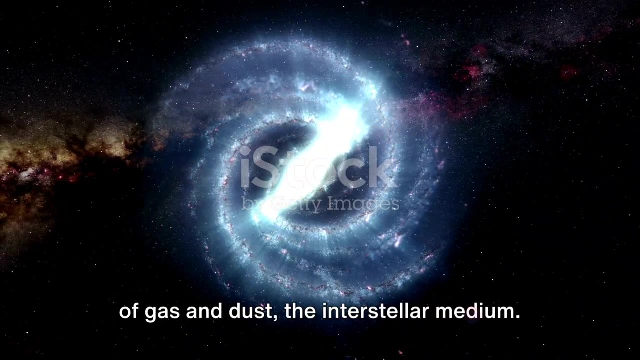 The young, the old, the brilliant and the dim. they all play their part in the cosmic dance that shapes our galaxy. Each star, whether young or old, plays a vital role in the dynamic tale of our galaxy. Between the stars lies a vast reservoir of gas and dust: the interstellar medium. 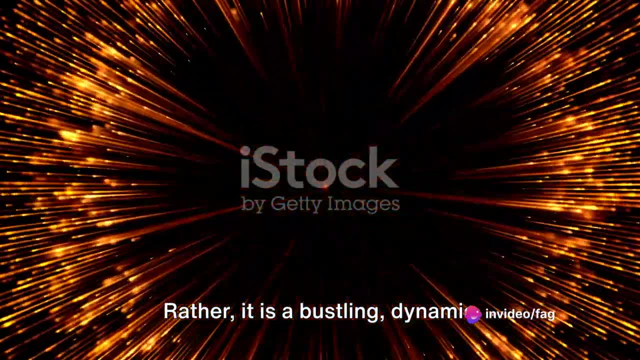 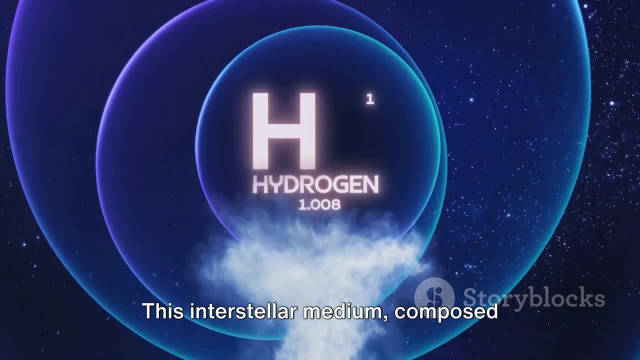 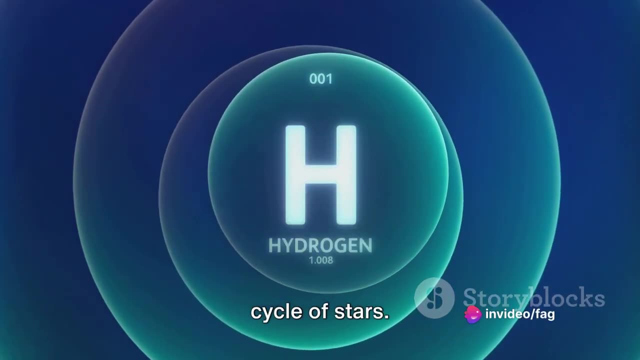 This seemingly empty space is far from inactive. Rather, it is a bustling, dynamic environment where the raw materials for new stars are found. This interstellar medium, composed primarily of hydrogen gas, along with trace amounts of helium and heavier elements, plays a pivotal role in the life cycle of stars. 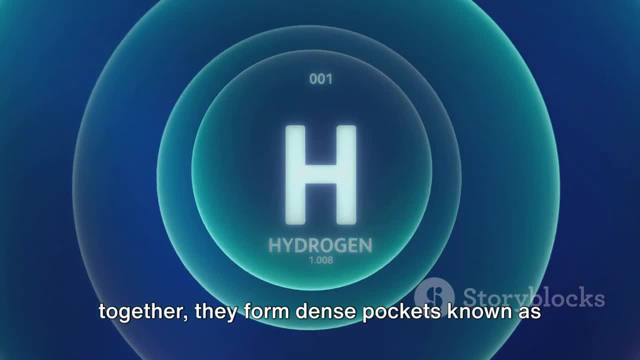 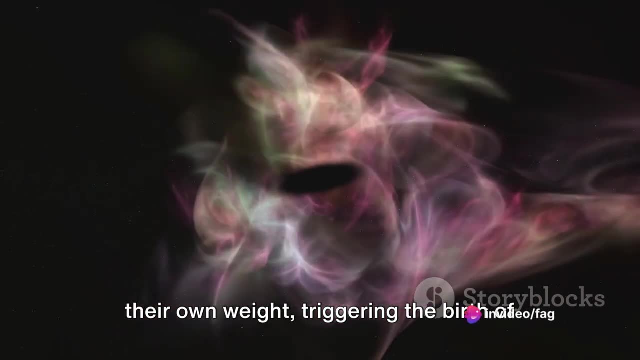 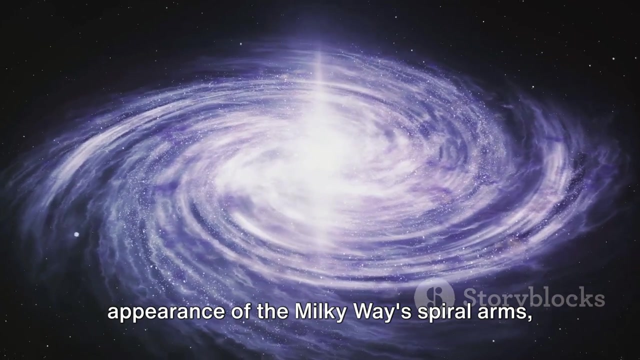 As gravity pulls these gases and dust together, they form dense pockets known as molecular clouds. Over time, these clouds collapse under their own weight, triggering the birth of new stars and planetary systems. The interstellar medium also shapes the appearance of the Milky Way's spiral arms. 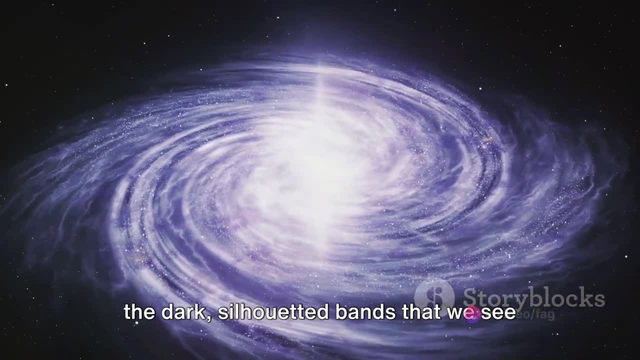 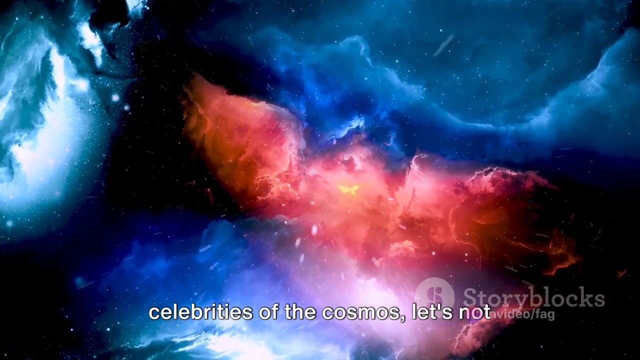 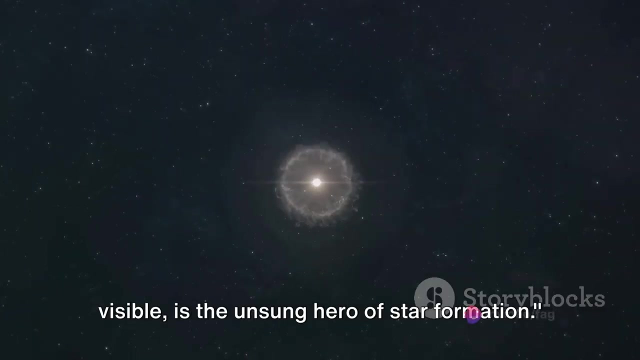 as its dense clouds block light and create the dark silhouetted bands that we see across our galaxy's disk. So, while the stars might be the celebrities of the cosmos, let's not forget about the essential supporting actor. This interstellar medium, although less visible, is the unsung hero of star formation. 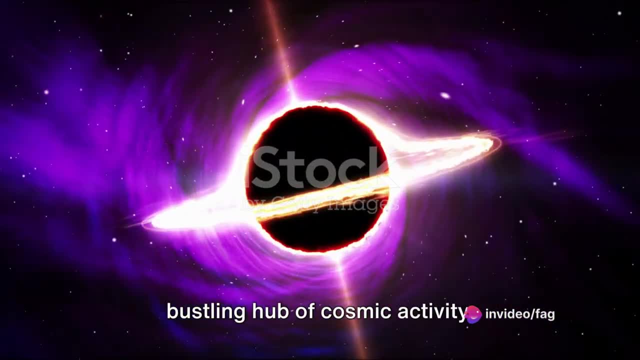 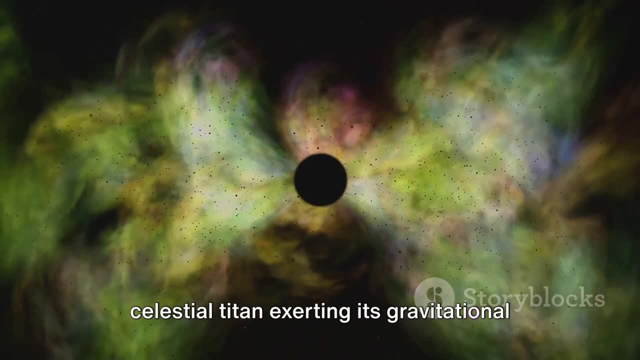 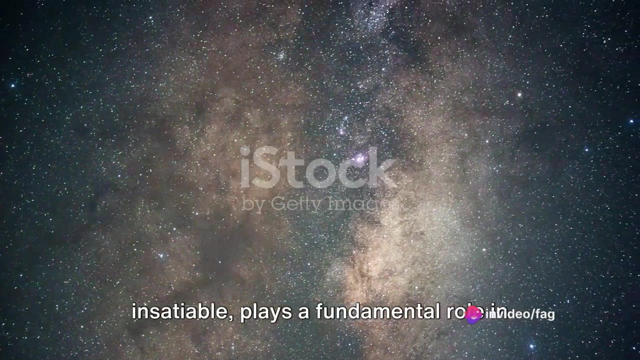 At the heart of our galaxy lies a bustling hub of cosmic activity. Located in this dense central region, we find a supermassive black hole, a celestial titan exerting its gravitational influence over the stars that dare to orbit too close. This black hole, while seemingly insatiable, plays a fundamental role in the Milky Way's life cycle. 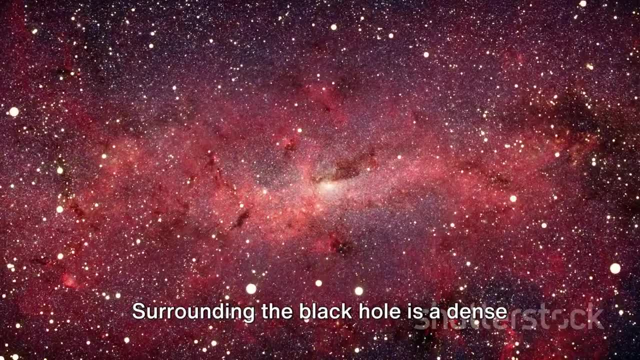 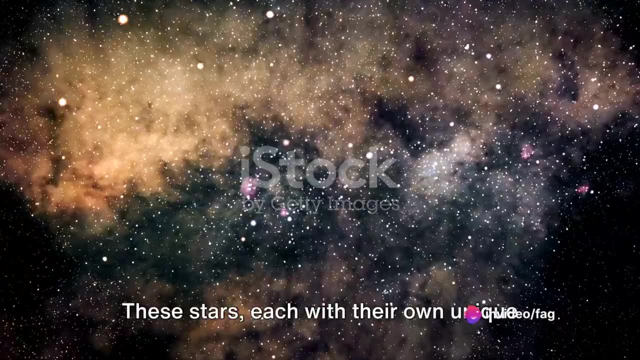 shaping its structure and dynamics. Surrounding the black hole is a dense cluster of stars, their light twinkling in the darkness like a city's skyline at night. These stars, each with their own unique story, contribute to the intricate dance of the Milky Way. 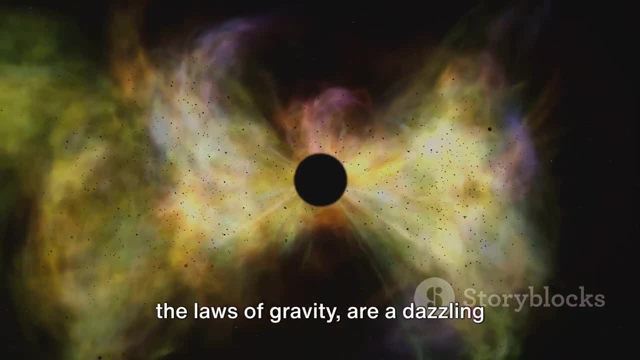 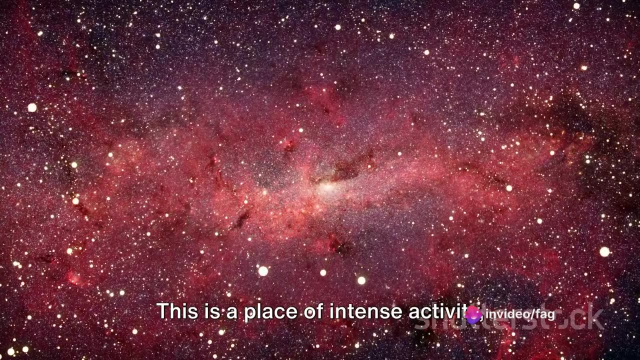 Their dynamic interactions, governed by the laws of gravity, are a dazzling spectacle of cosmic choreography. but this is not a tranquil scene. This is a place of intense activity, where stars are born, live and die, where gas and dust swirl in a constant chaotic ballet. 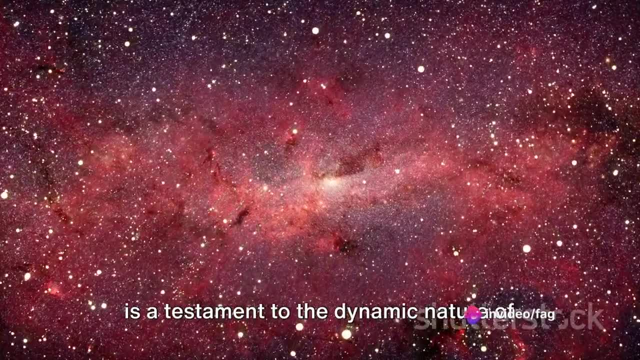 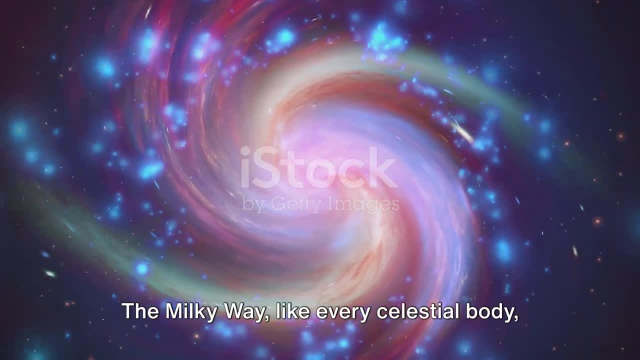 This galactic center, a hive of activity, is a testament to the dynamic nature of our galaxy. Our galaxy's story is one of change and evolution spanning billions of years. The Milky Way, like every celestial body, has not been static. 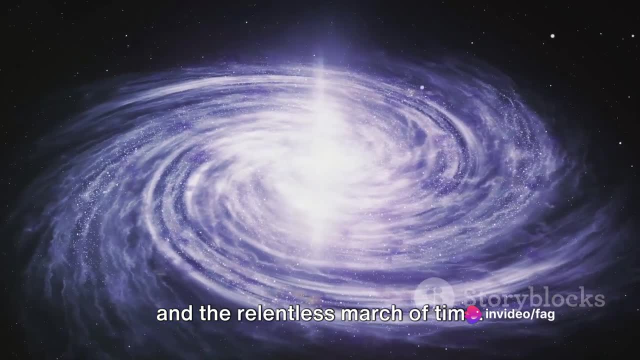 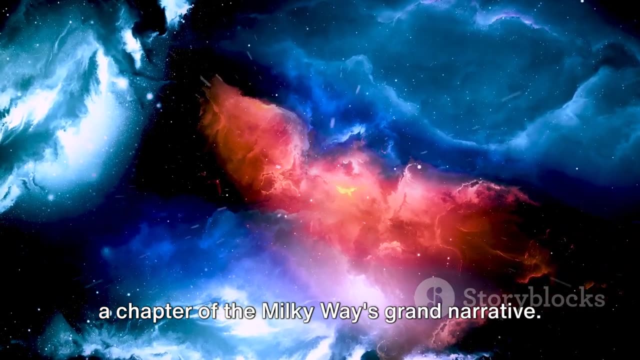 It has evolved, shaped by cosmic forces and the relentless march of time. The spiral arms, the central bulge, the halo of ancient stars. each element tells a chapter of the Milky Way's grand narrative. Over the eons, galaxies like ours have been sculpted by the dynamic interplay of matter and energy. 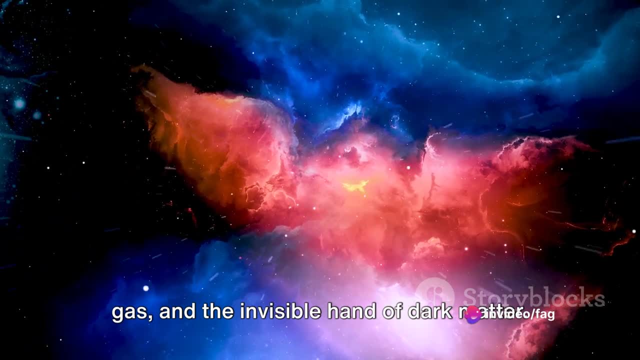 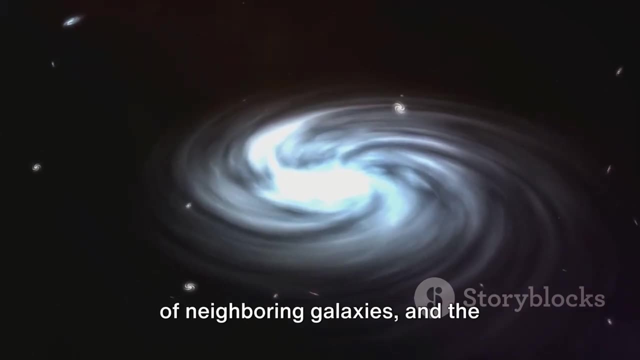 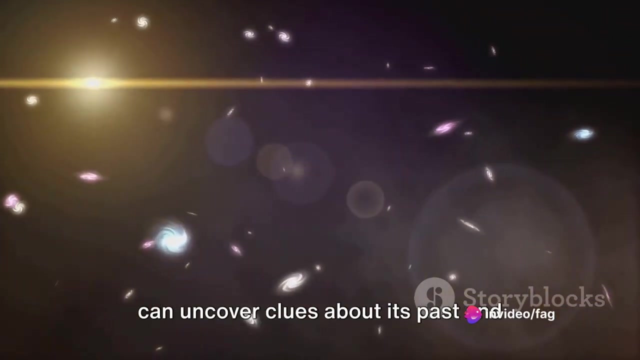 the dance of stars and gas and the invisible hand of dark matter. Their forms have been molded by the birth and death of stars, the gravitational tug of neighboring galaxies and the mysterious forces that drive cosmic expansion. By observing the Milky Way, astronomers can uncover clues about its past and predictions for its future. 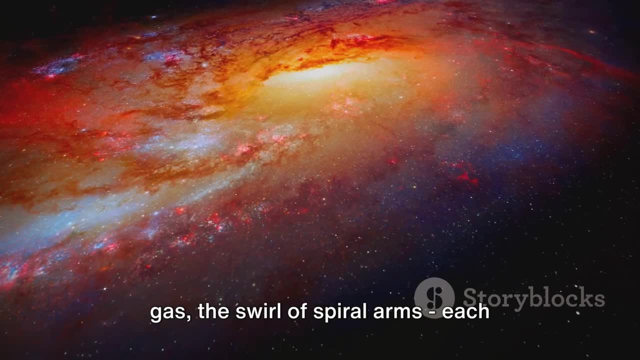 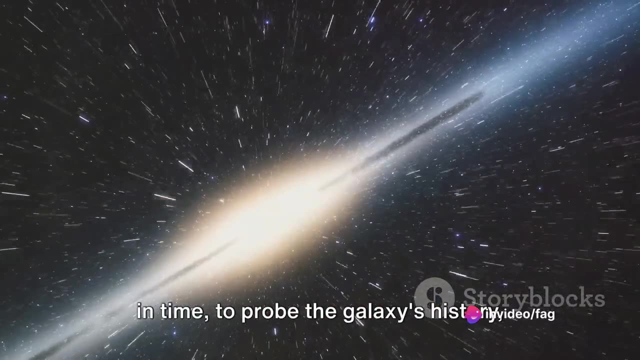 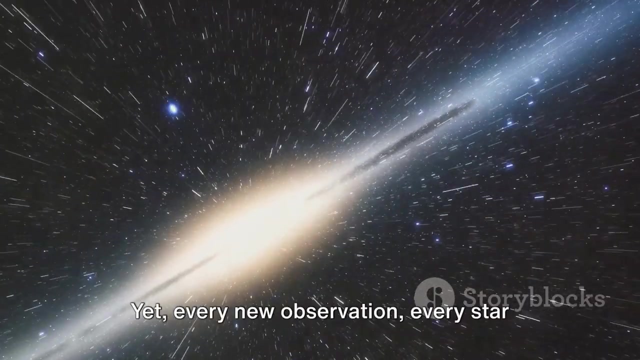 The distribution of stars, the motion of gas, the swirl of spiral arms: each provides a piece of the puzzle. These observations allow us to peer back in time, to probe the galaxy's history and to forecast its destiny. Our understanding of the Milky Way's evolution is far from complete.